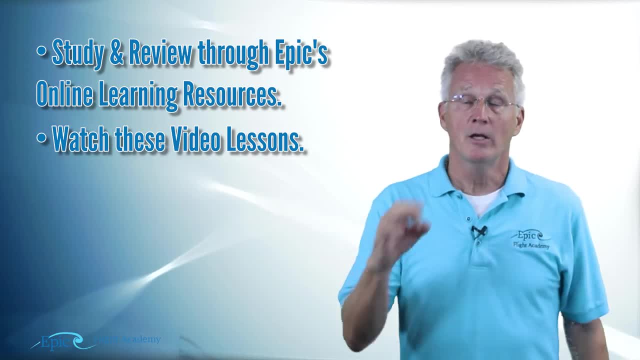 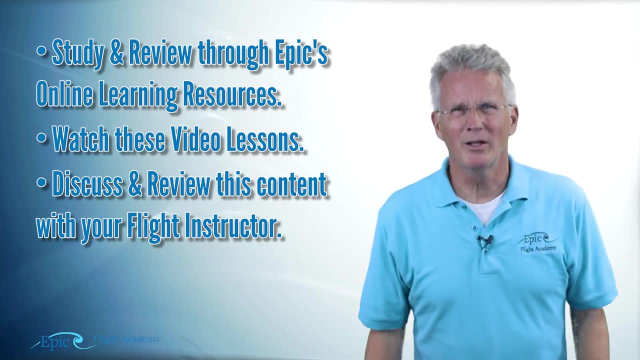 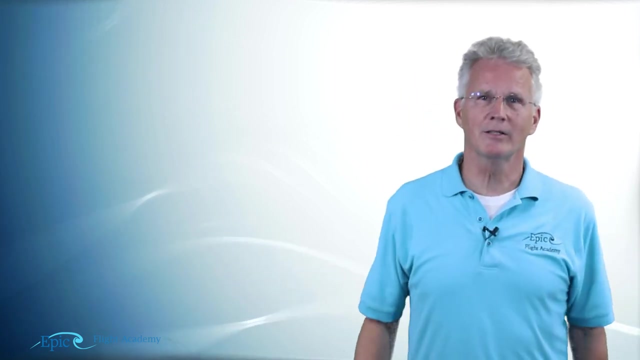 parallelize the course. Number three: you're going to use these videos to parallelize the course, The content in that course, And number three: be sure to review all of this with your flight instructor. Now, what about that Coriolis force? It keeps turning to the right. Yeah, take a look. 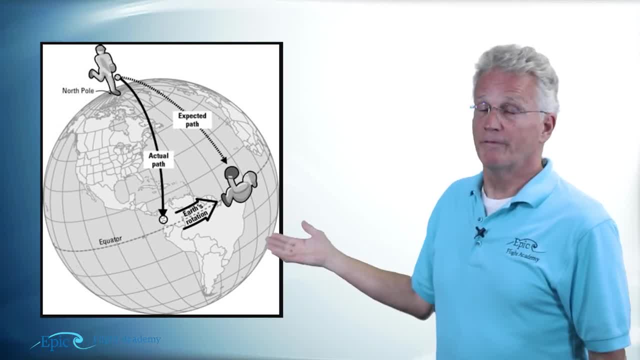 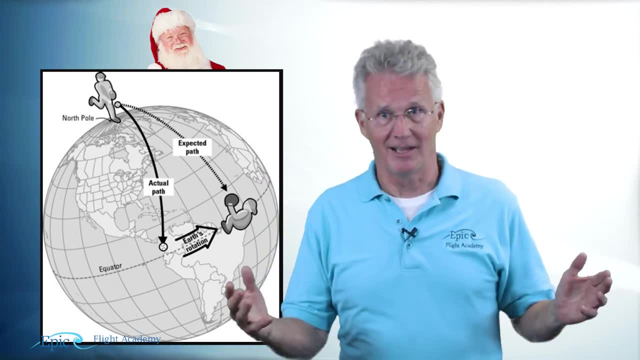 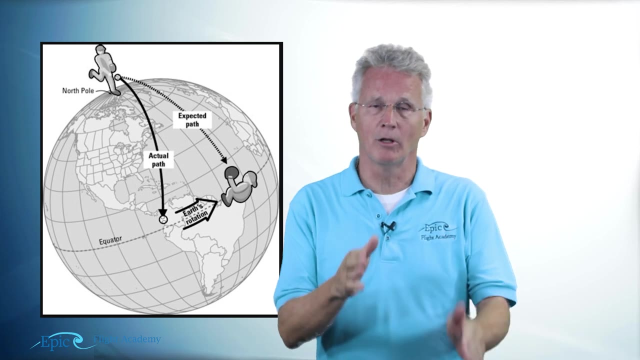 at this diagram here. Let's imagine we were visiting Santa Claus and we're standing up here at the North Pole and that year for Christmas Santa gave me a soccer ball. Now I'm standing up here at the North Pole and I am going to kick that soccer ball straight south. 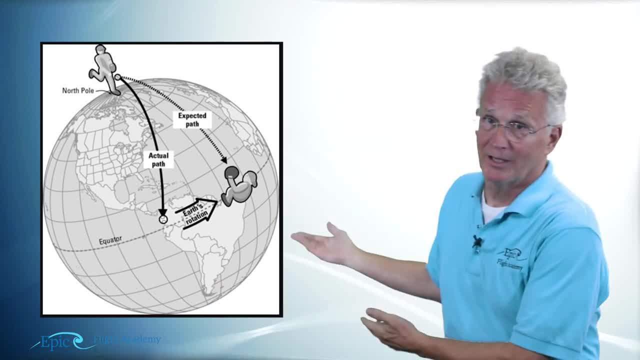 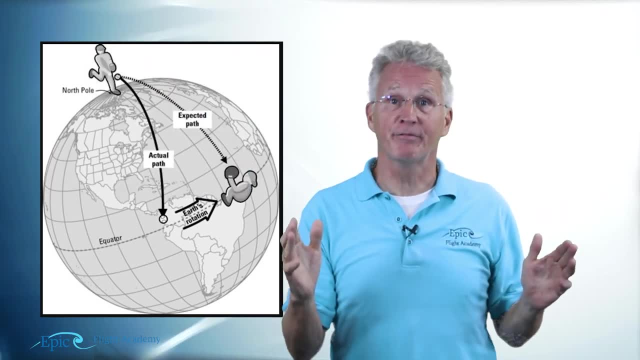 Now I've got a pretty good soccer kick and, as you can see in my diagram, I'm kicking it all the way to Brazil. You what? Yeah, that's right, All the way to Brazil, If the planet were not rotating. 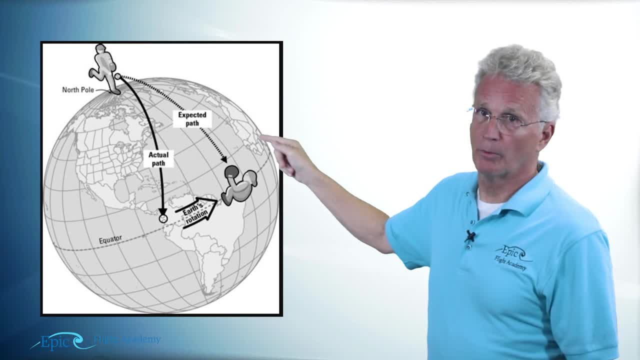 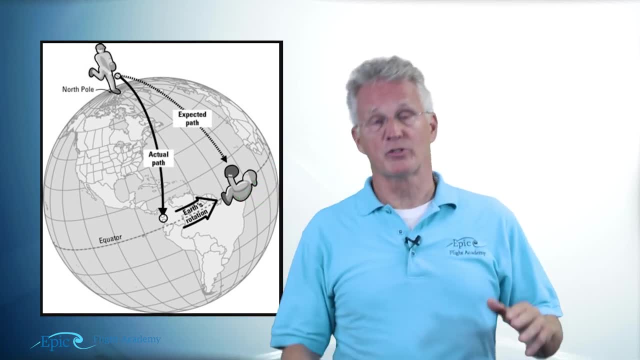 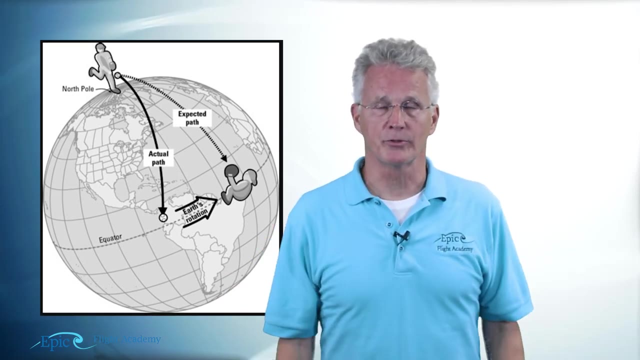 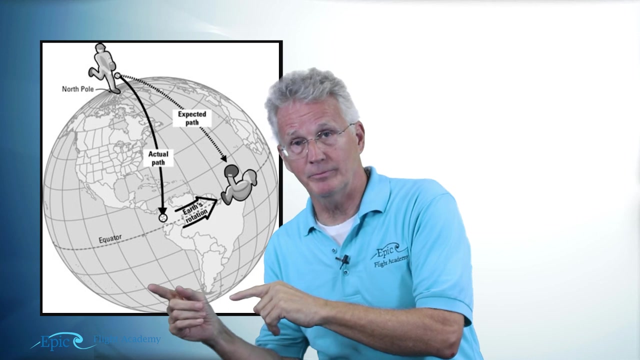 that soccer ball would come straight south from the point I kicked it all the way to Brazil. But in fact, of course, the Earth is rotating and this brings about the Coriolis force. Now it's important to understand which direction the Earth rotates. If you look at the globe here, 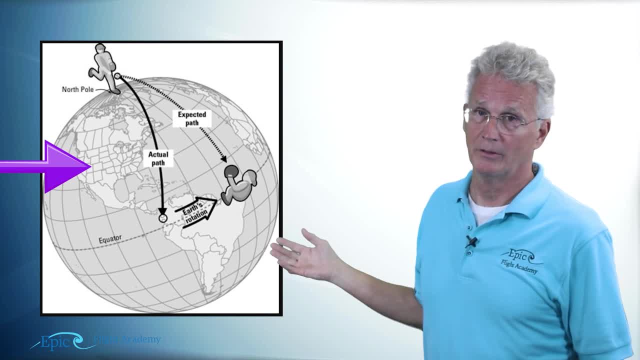 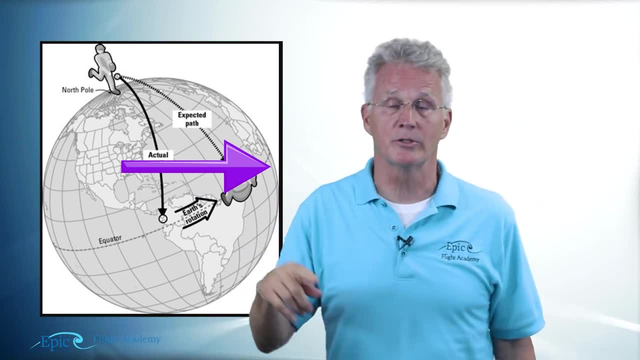 you can see the North American continent moving toward England or Europe. Okay, that's the direction of the Earth. Now, if you look at the globe here, you can see the North American continent moving toward England or Europe. Okay, that's the direction of the Earth. 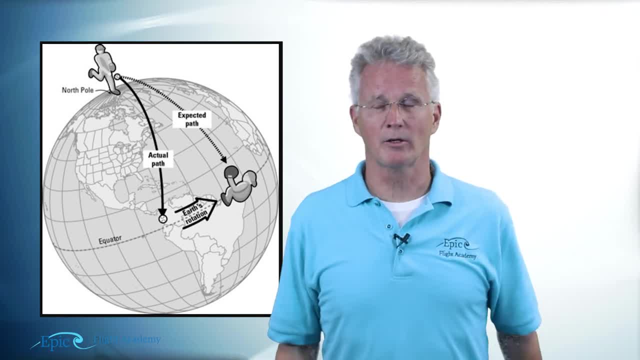 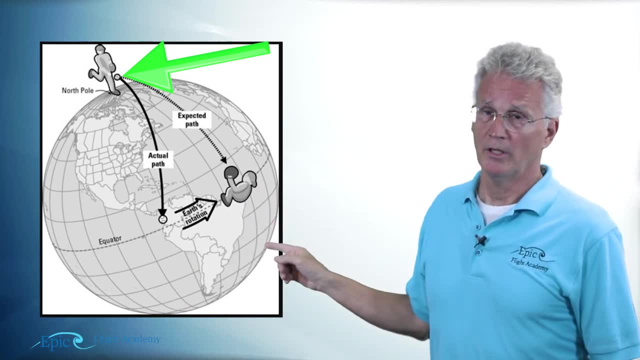 Now, if you look at the globe here, you can see the Earth's rotation. Now let's go back to that soccer ball. I'm standing up by Santa Claus's house and I'm going to kick that soccer ball to Brazil. Now the soccer ball is still going straight. 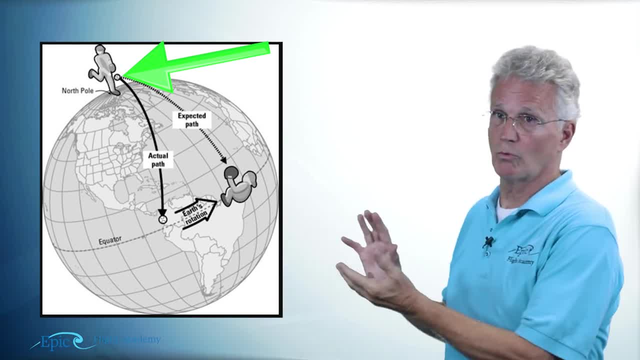 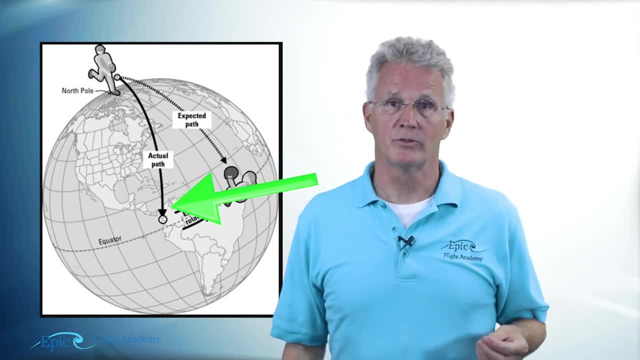 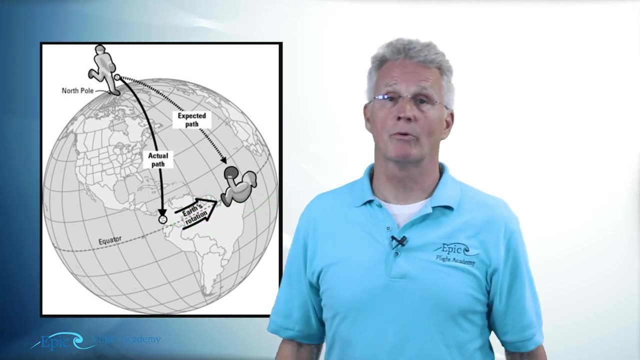 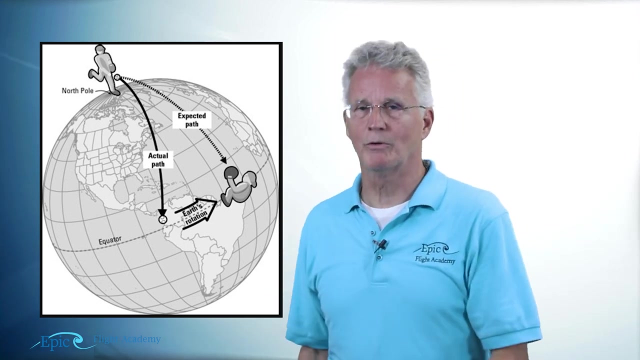 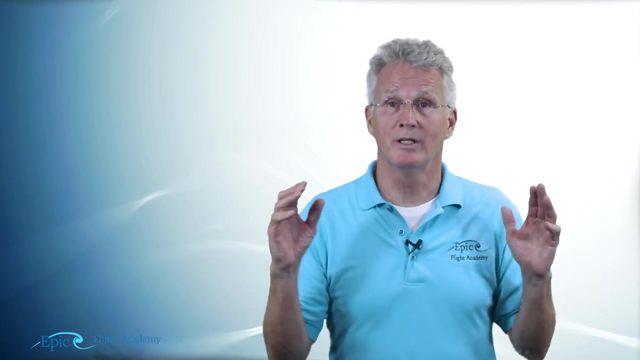 south, but because the Earth is rotating underneath of it. look where it lands. That land out near Ecuador. force turns it to the right. The soccer ball is going straight, but its path is curved to the right because of rotation. Now let's imagine if we were in the South Pole and we're standing out. 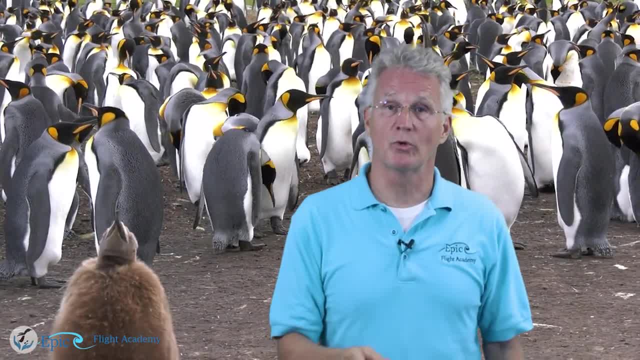 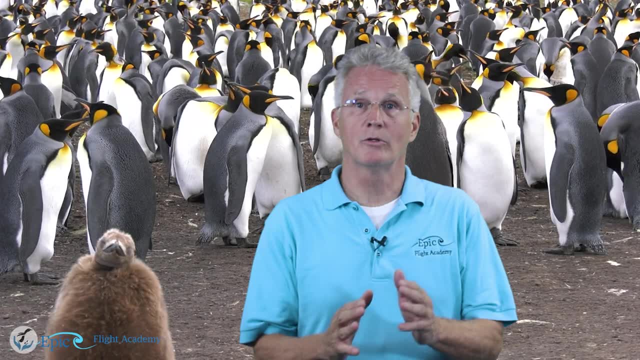 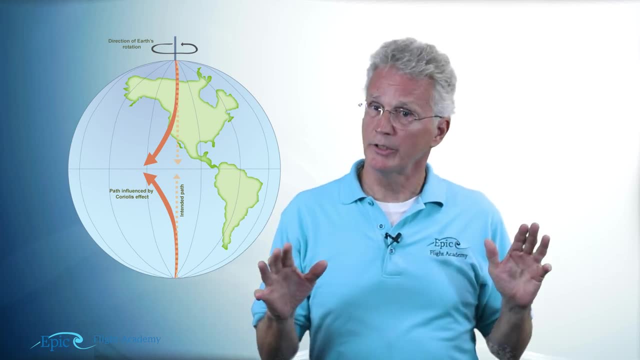 there amongst the penguins, and we're going to kick this soccer ball straight north. because of the Earth's rotation, Coriolis would turn it to the left. But let's not confuse ourselves, since, at least initially, we're going to do most, if not all, of our flying in the northern hemisphere. 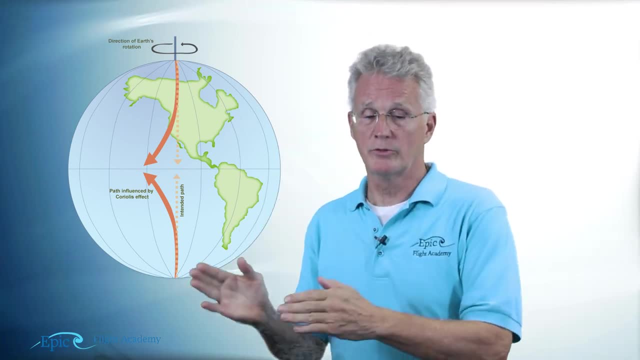 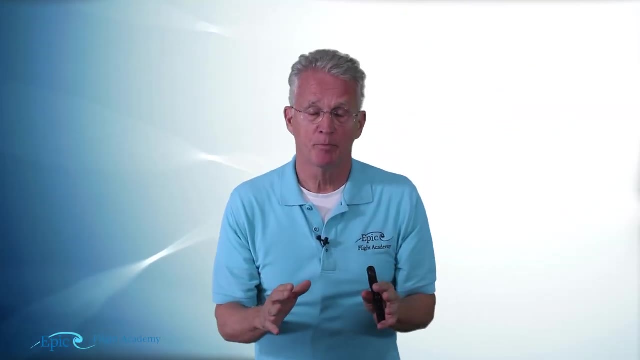 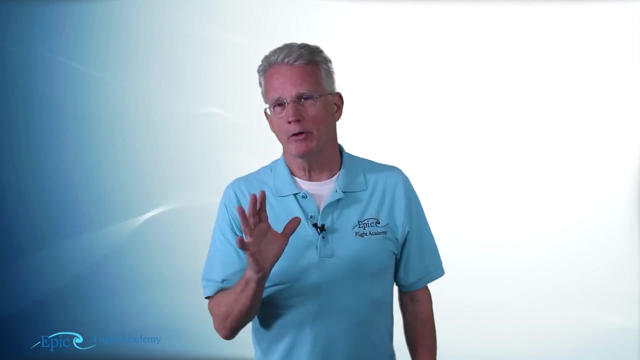 We'll just stay focused on the fact that Coriolis turns to the right. Now. that is the Coriolis effect talking about air moving toward the equator. Now the Coriolis effect also affects air moving along the equator. 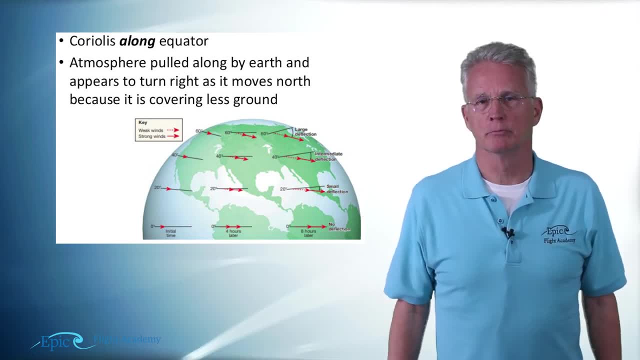 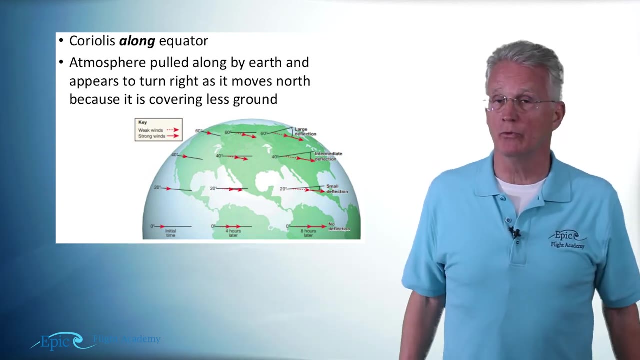 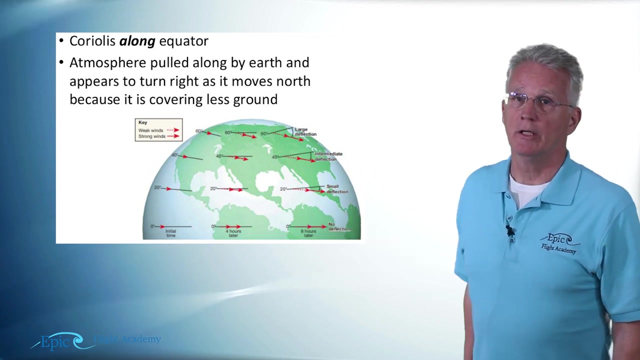 The atmosphere is pulled along by the Earth and appears to turn right as we move north, because, as the atmosphere is being pulled along parallel to the equator, as we move north we're covering less and less ground. You can see an example of that here in this diagram, Now also in this. 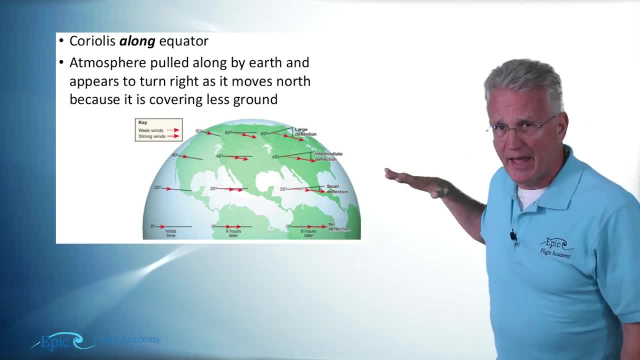 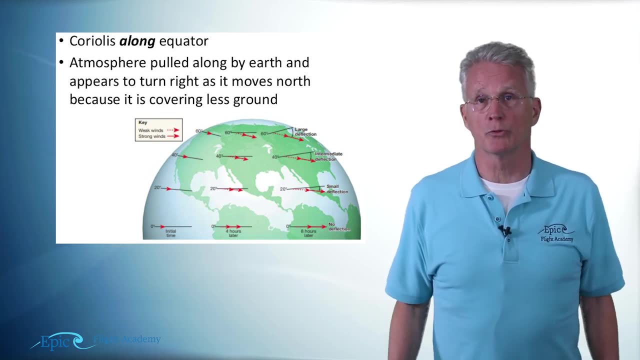 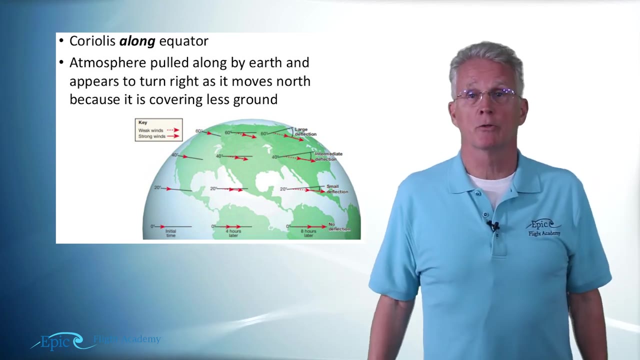 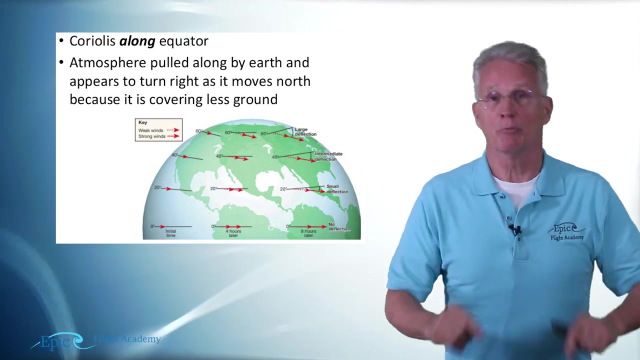 diagram you can see that that effect becomes stronger the closer we get to the poles. Why? Because there is less and less surface area to cover as we move closer and closer to the poles. That's called the conservation of angular momentum, and I know that sounds like a big concept. but 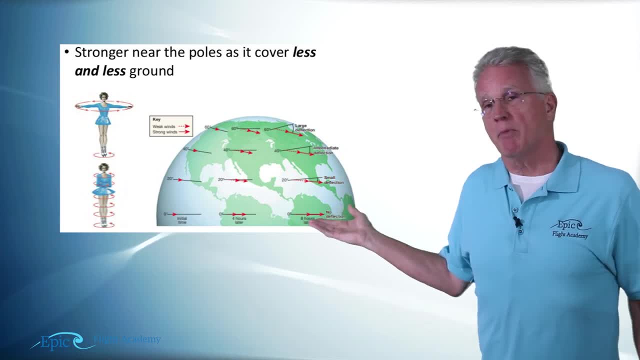 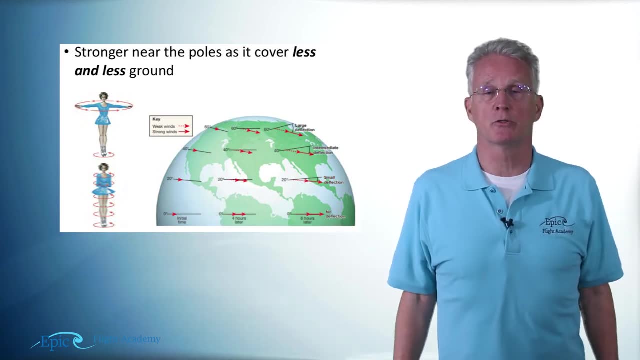 it's really just the same as this dancer, And I think many of us have experienced this As we're spinning around in a circle. when the dancer puts her arms out, she tends to move slower. That would be the atmosphere closer to the equator. 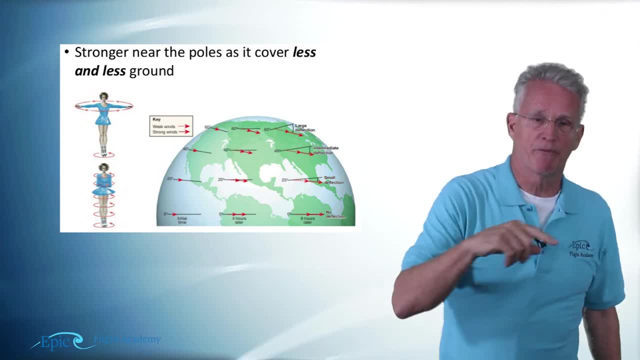 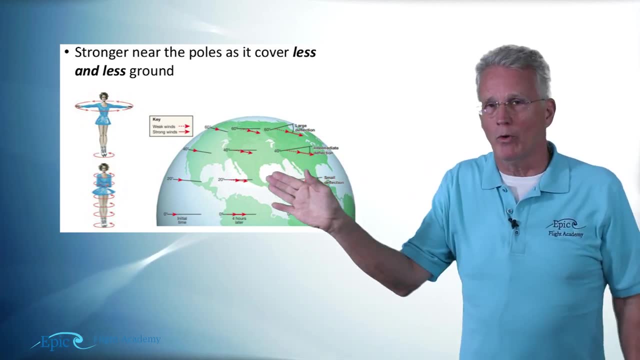 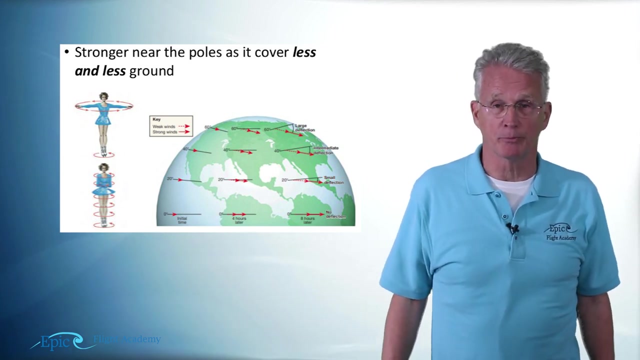 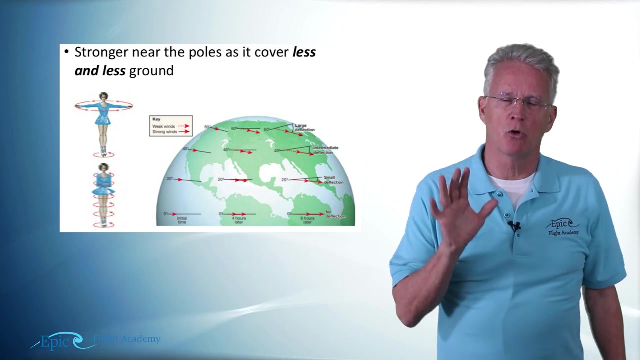 As the dancer pulls her arms in, she spins faster. That would be the atmosphere as it is drifting north toward the pole and that Coriolis effect turns it to the right more and more the closer we get to the poles. So so far we've talked about the Coriolis effect and its effect on the horizontal movement of air. 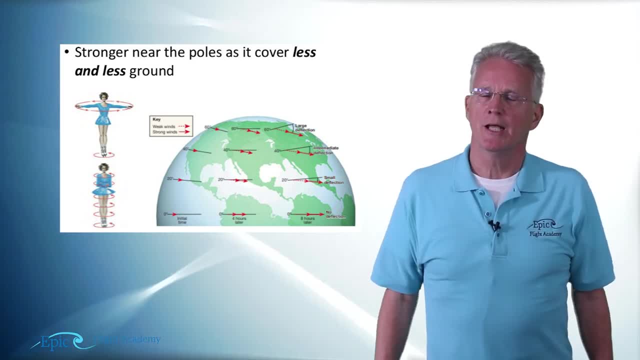 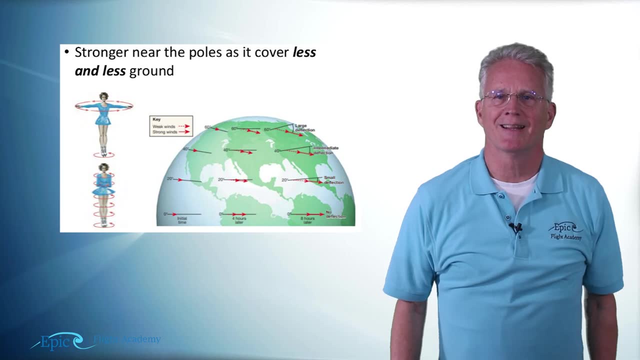 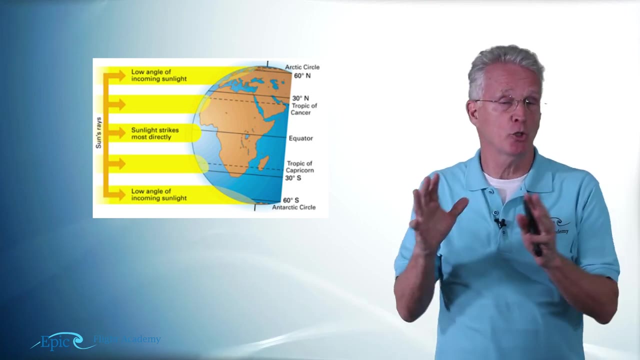 Now. secondly, when it comes to global circulation, it's just as important to understand the vertical movement of air. Now, in order to understand that, let's begin with this diagram, where we look at how the Sun heats the Earth's surface. Notice in the diagram I want to call your attention to. 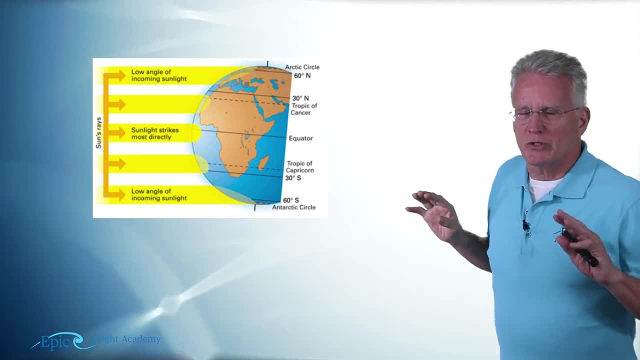 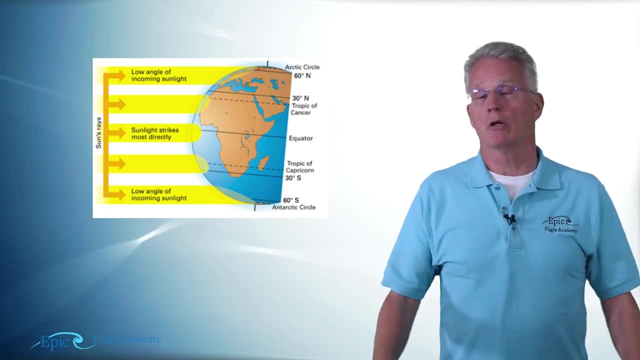 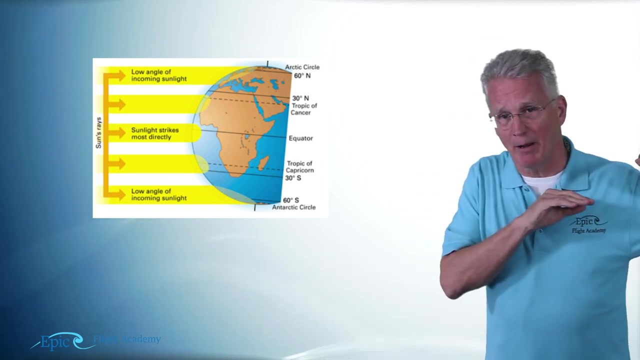 two key things. Number one: the Sun's rays are hitting the Earth's surface at a different angle. You can see closer to the equator, the Sun is more directed And as we move towards the pole, that same amount of incoming sunlight. 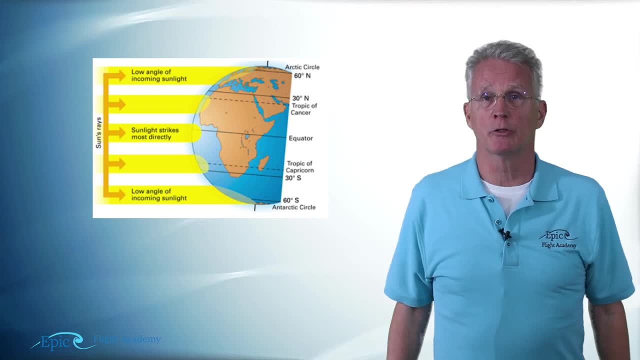 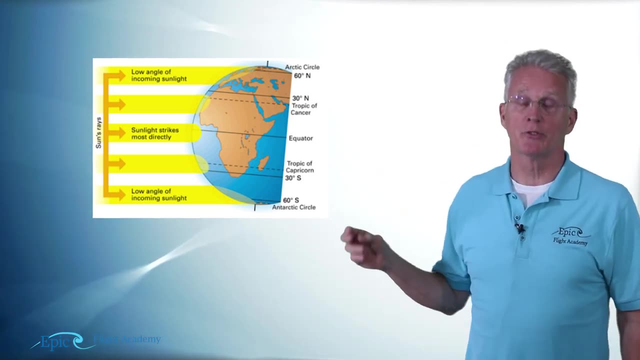 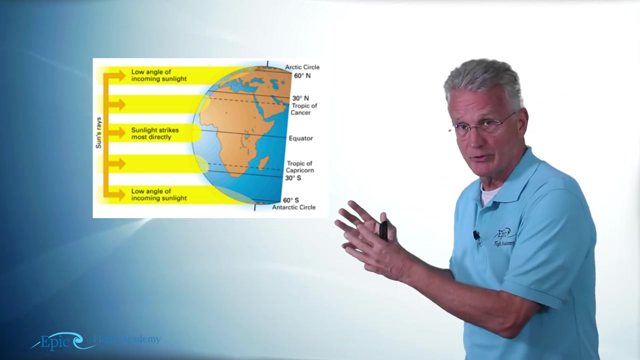 is spread over a larger and larger surface area, So of course the planet gets cooler near the poles Now. the second thing to notice is that the Sun will heat the Earth differently depending upon the surface. Land masses will heat and cool faster. 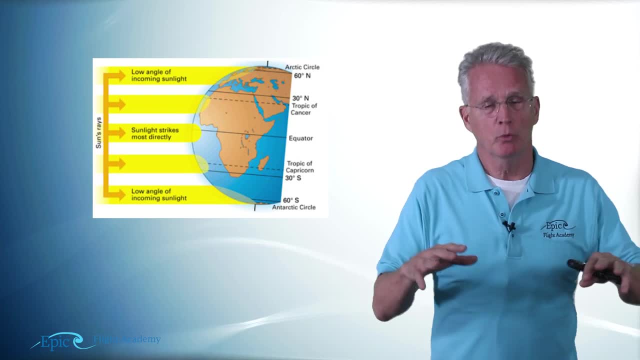 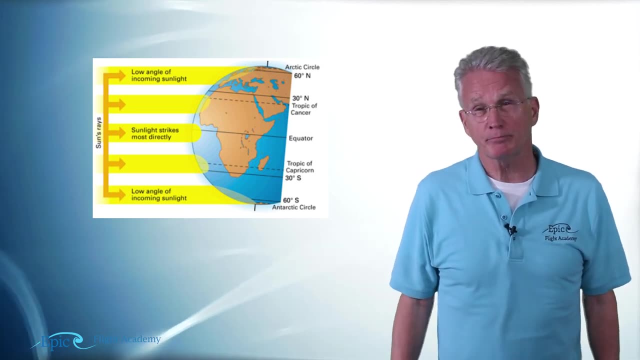 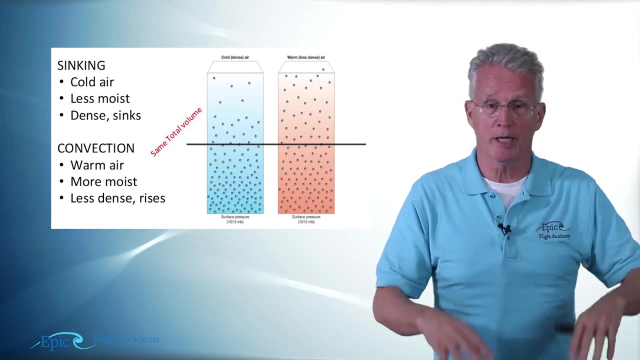 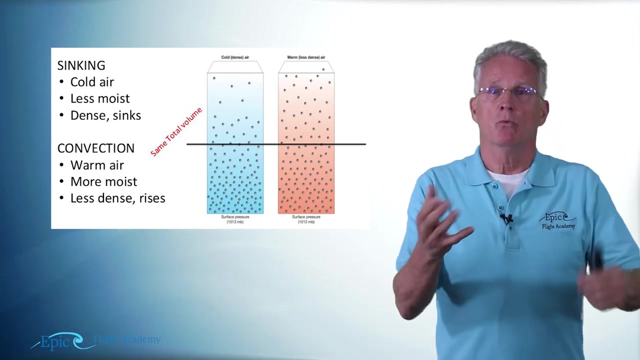 Water, such as the oceans, will heat and cool slower. This will affect the vertical movement of air. Now we know that sinking air is cooler. its less moist and more dense. Warm air is more moist and tends to rise. Well, it you ever wonder exactly why that happens, I want. 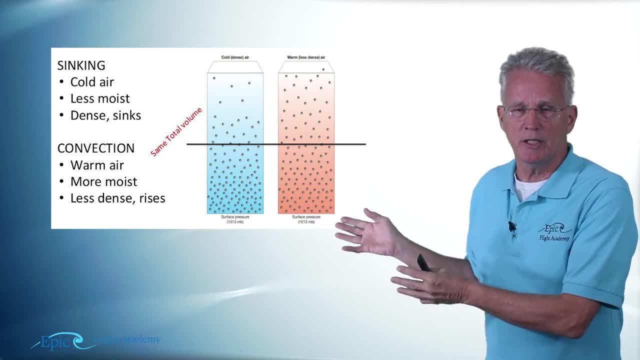 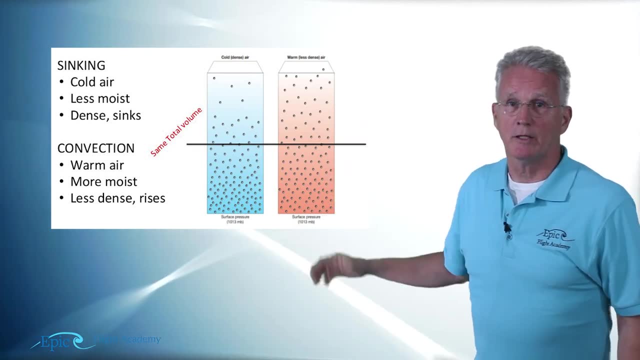 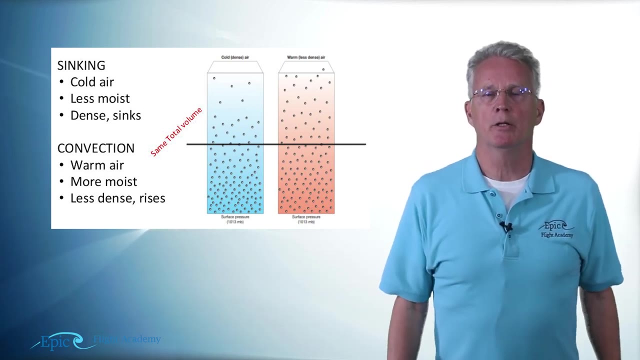 you to look at this diagram to explain why this happens. I want you to take a look at this diagram and see in both cases, the blue column and the orange or red colored column, we have theoretically the same volume of air, but notice, because the blue column 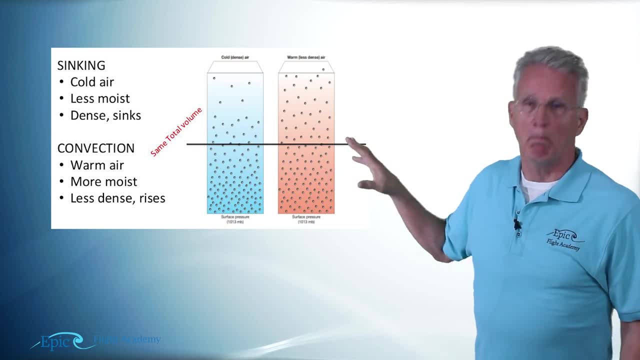 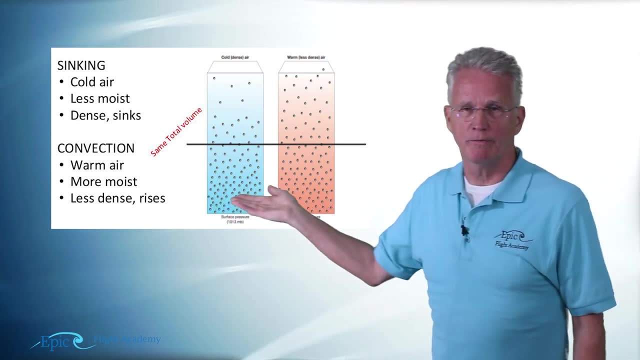 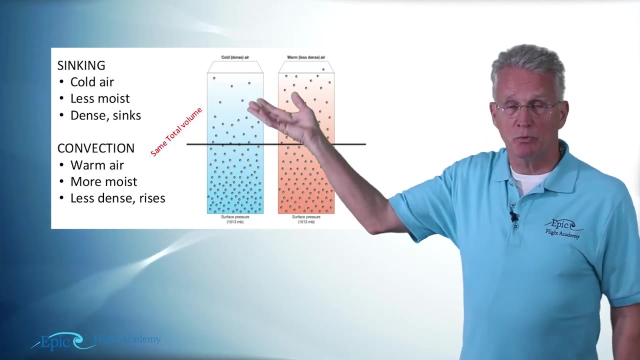 is cooler. more of that air is settling to the bottom. notice: we've outlined here the halfway point in these two vertical columns, so if you can imagine they have the same volume. you see how in the red column it's more spread out and in the blue column it's more condensed. 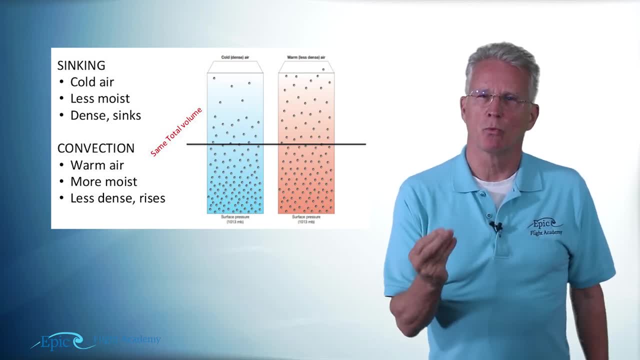 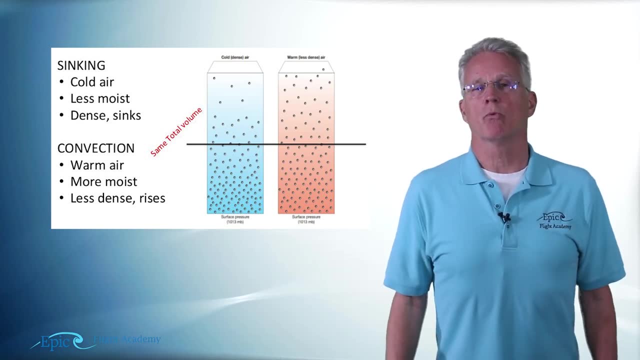 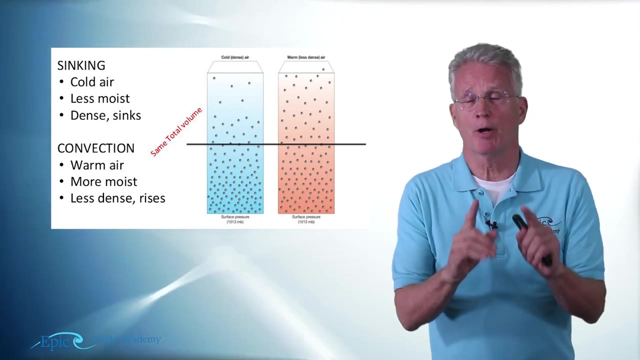 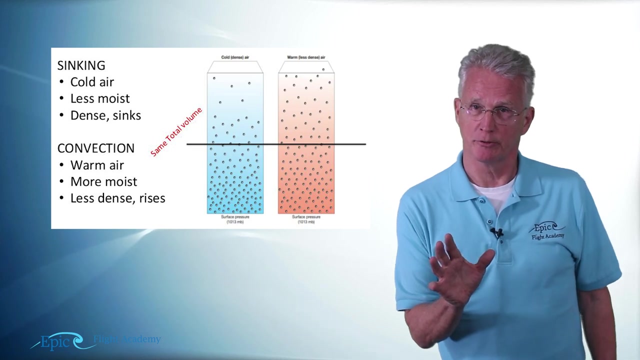 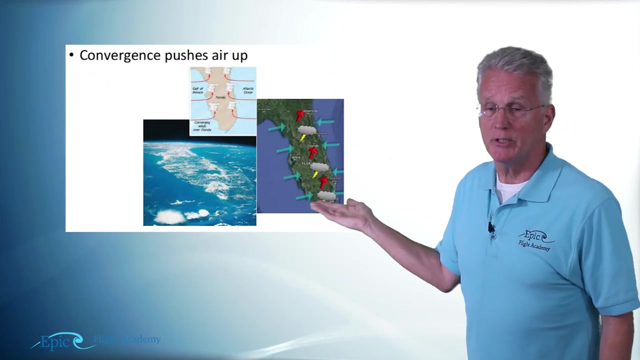 near the bottom, and this is what we mean by cold air sinking and warm air rising. that warm air rising we know as convection, convection, convection. the final part of the vertical movement of air that we need to understand is convergence. now remember we just talked about convection. this is convergence and you can see in these pictures. 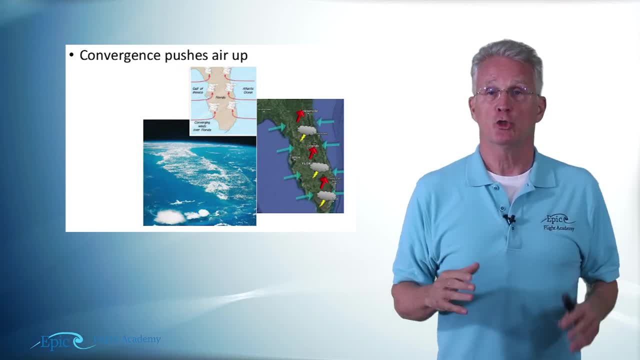 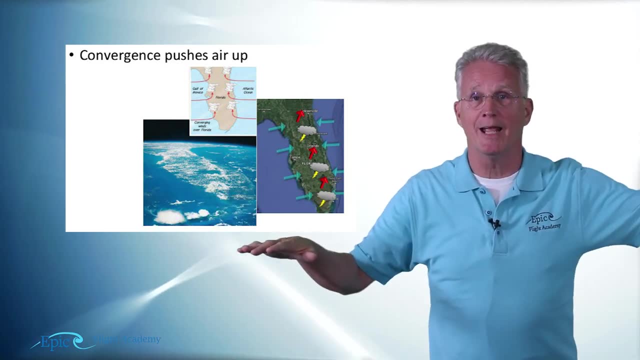 an excellent example of convergence just happens to be florida itself, as air is moving in from the atlantic and in from the gulf of mexico. this air is moving in from the gulf of mexico. this air is moving in from the gulf of mexico and in from the gulf of mexico. 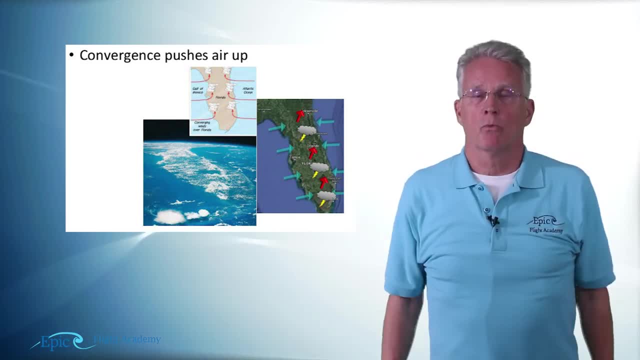 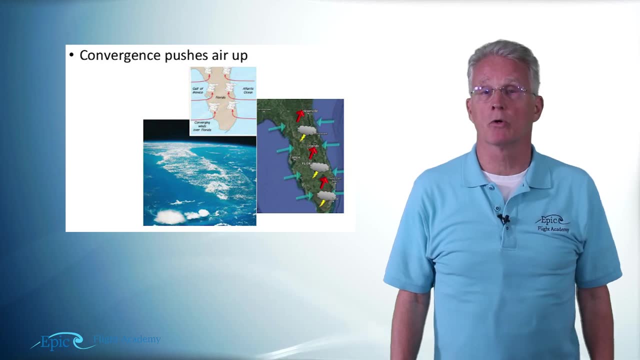 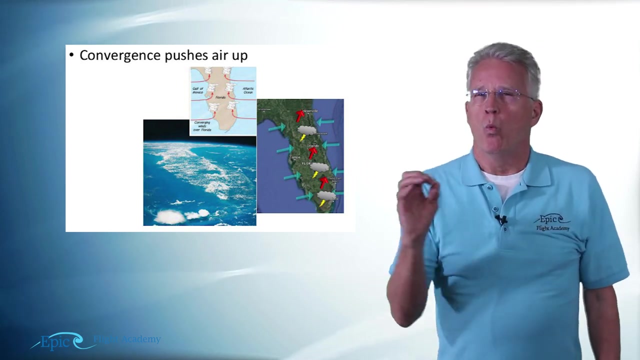 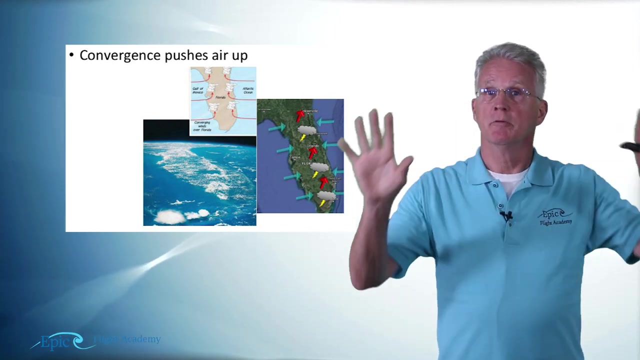 and in from the gulf of mexico, converges bumps into each other and rises Vertical movement of air. So thus far we have talked about the horizontal movement of air and the vertical movement of air. Now one more key thing to understand before we discuss atmospheric circulation. and then it's all going to come. 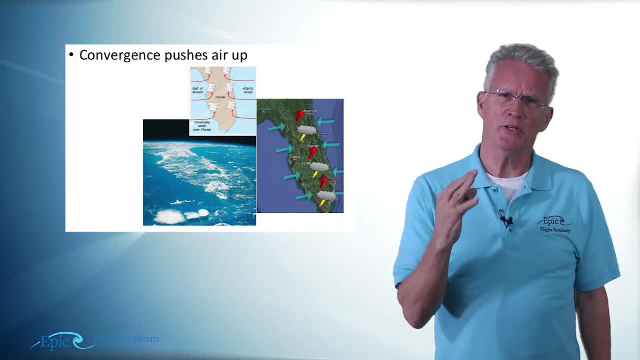 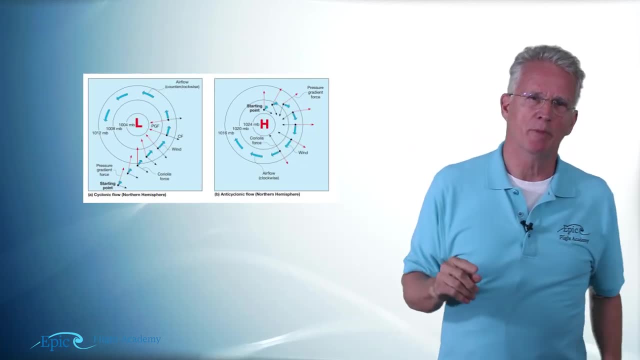 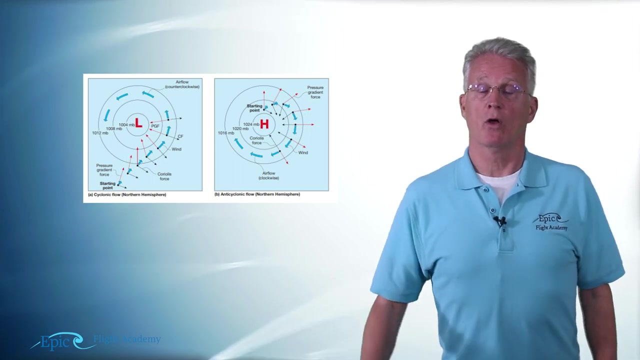 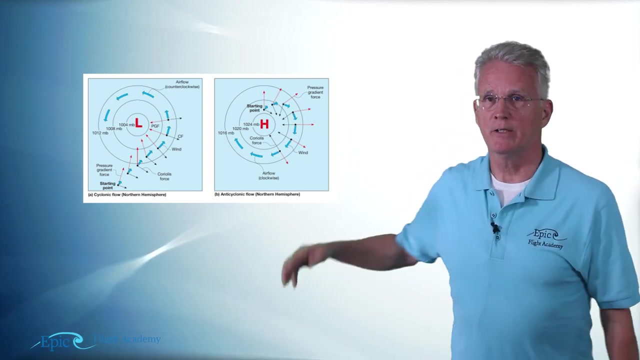 together and click. And this third and final key is called PGF, or pressure gradient force. Now what does that mean? Remember, atmosphere will seek a balance, So it will flow from a high pressure and into a low pressure. If you take a look at our diagram here, you can see that the red line, 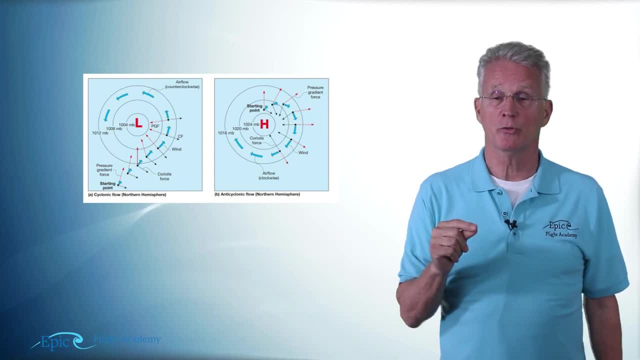 is the pressure gradient force, And if you take a look at the diagram here, you can see that the red line is the pressure gradient force. And if you take a look at our diagram here, you can see that the red line is the pressure gradient force, And it turns right in both cases. 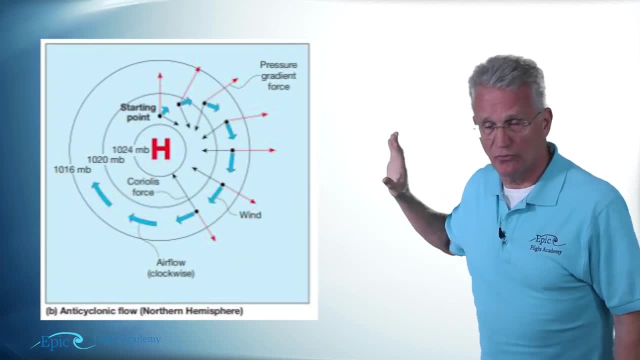 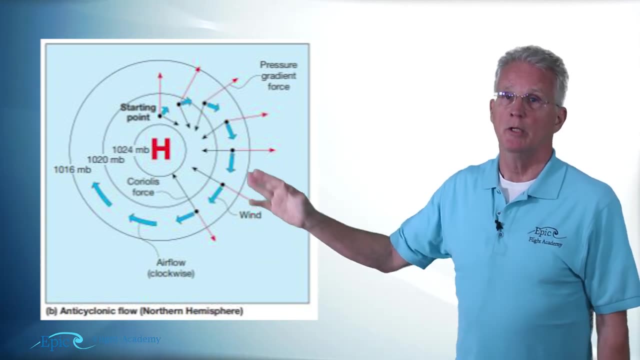 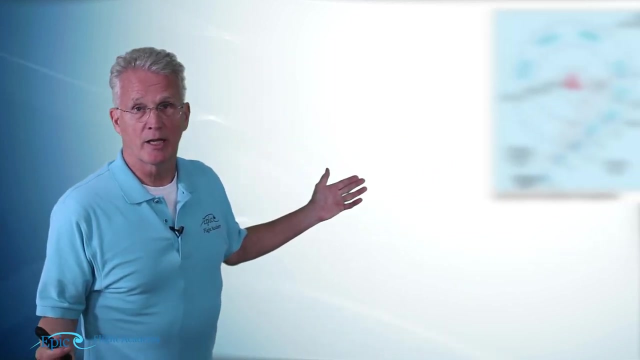 In the high pressure it's flowing away toward low pressure And you can see the red line, which is our pressure gradient force being turned to the right by Coriolis force. Now in the low pressure, it's the same thing. The red line is the pressure gradient force flowing into or 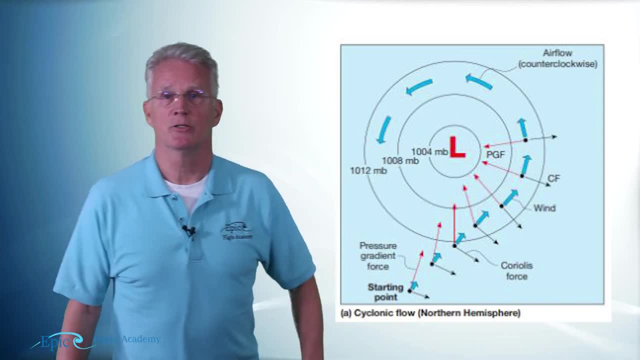 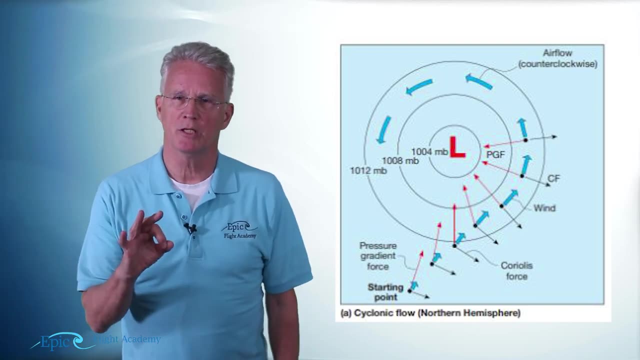 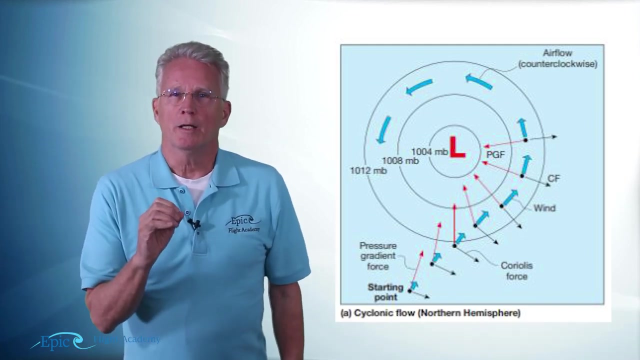 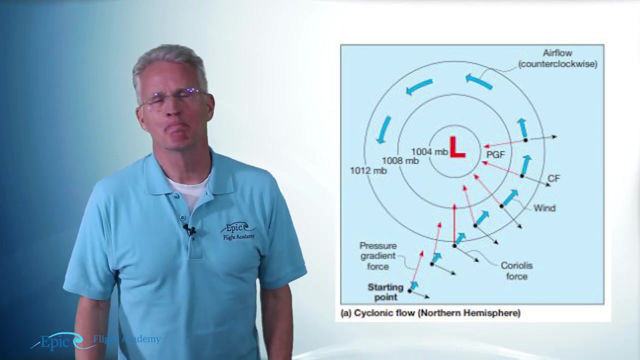 toward the low And again it is being turned to the right by pressure gradient force. So if we can put all three of these keys together- horizontal movement of air, vertical movement of air and pressure gradient- we are about to master an understanding of global circulation. 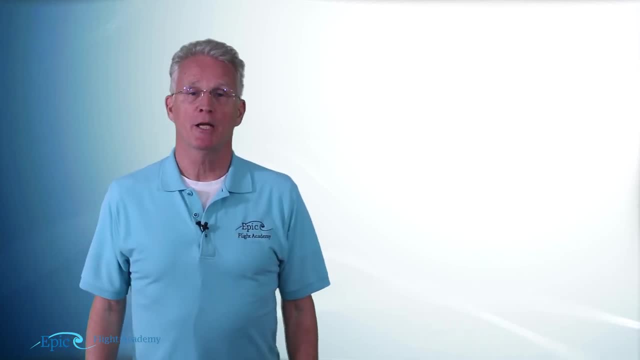 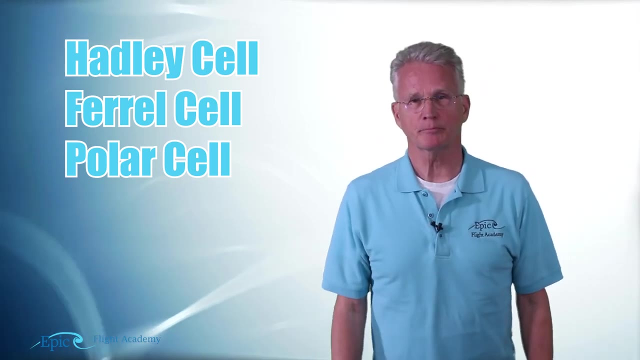 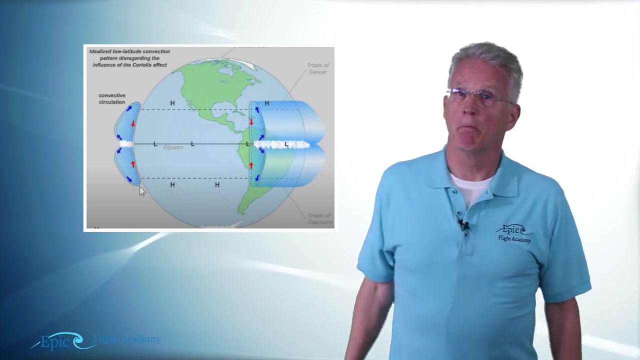 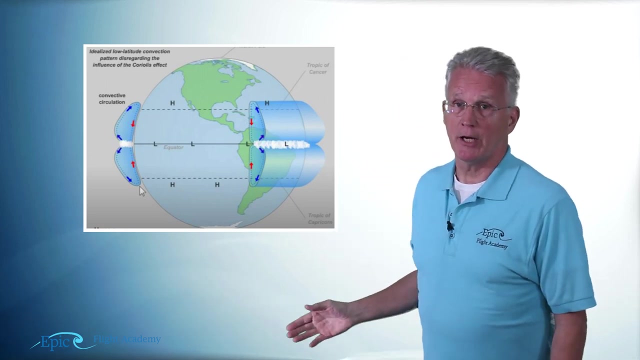 In global circulation. there are three major cells: the Hadley cell, the Ferrel cell and the polar cell. So let's start here with this diagram. We can see that the Earth is much warmer near the equator And again we know why, And you can see this air starts to rise And at some point it will. 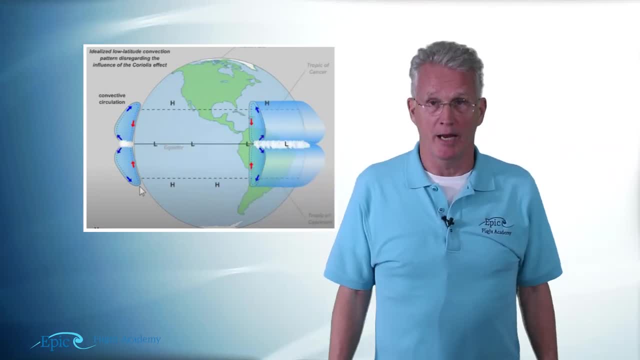 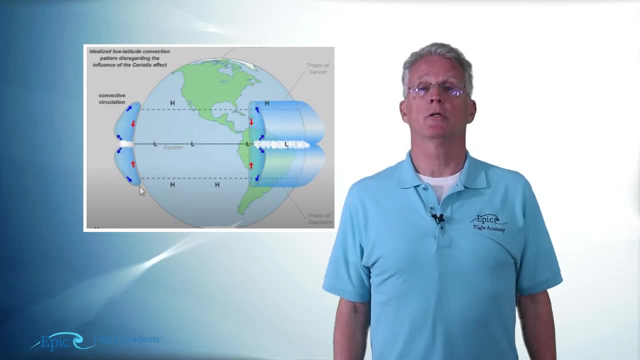 start to rise, And at some point it will start to rise, And at some point it will start to rise To diverge both north and south. Now, at what point will it stop rising? That, my friends, is the. 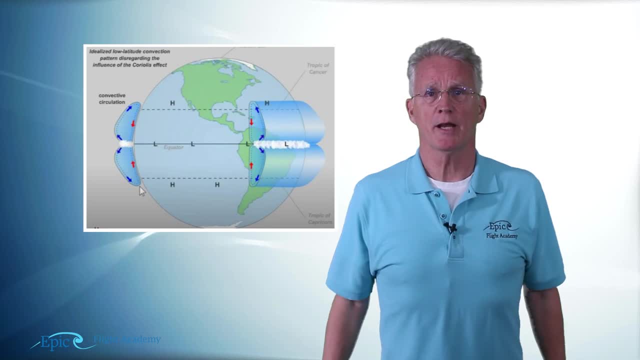 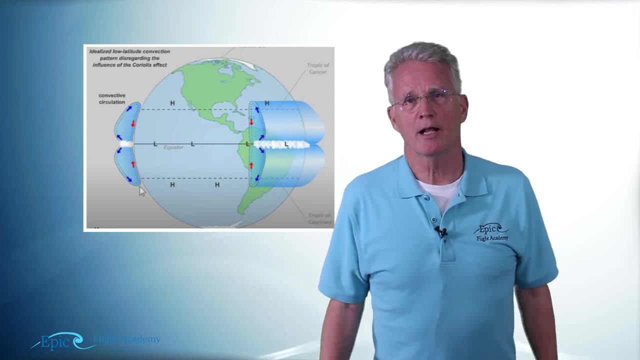 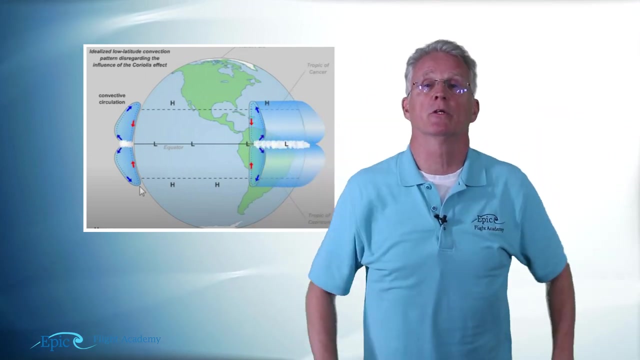 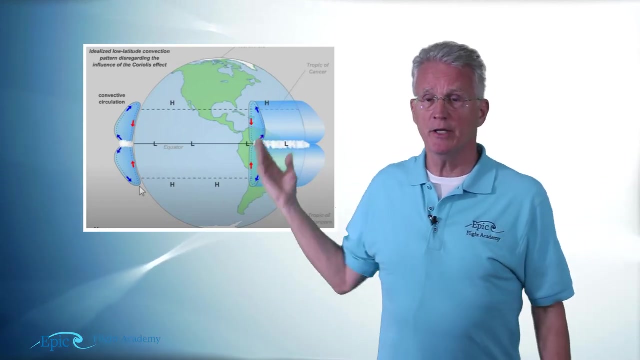 tropopause or the bottom of the stratosphere. The air will then proceed to the north, proceed to the south and, as it travels toward the pole, it starts to cool and will fall towards the surface of the equator approximately 30 degrees of latitude. Now, in this diagram, we are disregarding the Coriolis force. 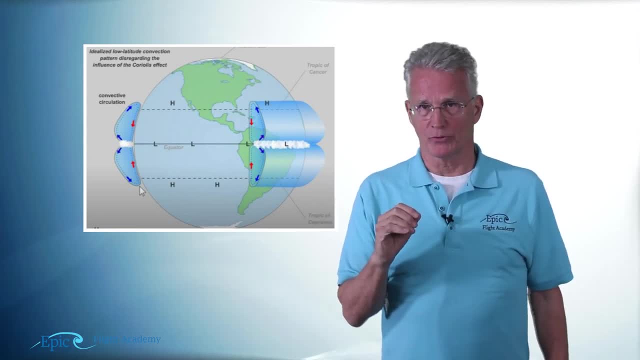 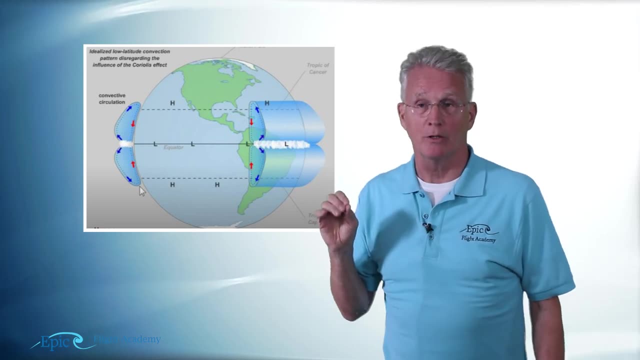 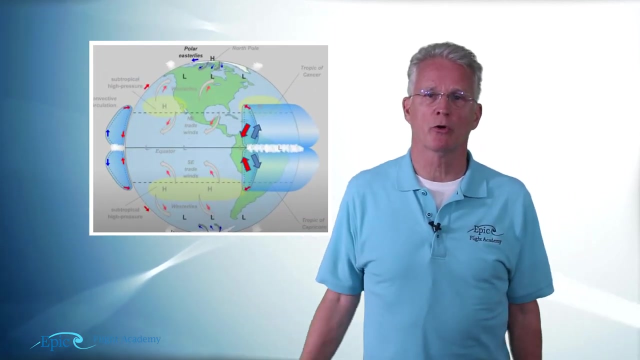 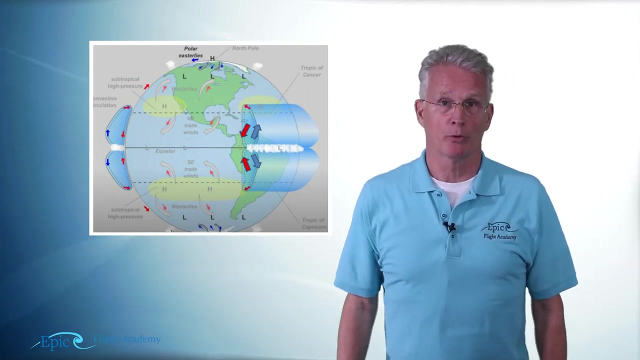 Now when we add Coriolis force, both north and south and along the equator, we can see in this diagram Coriolis force is turning the surface flow to the right, And that was the Coriolis coming from the pole toward the equator. 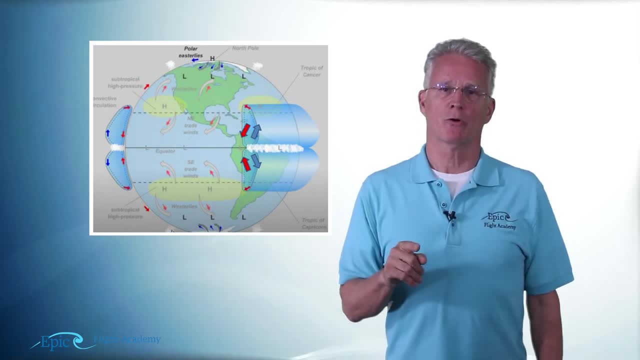 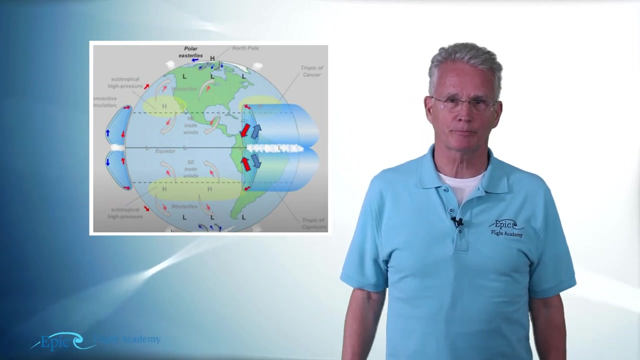 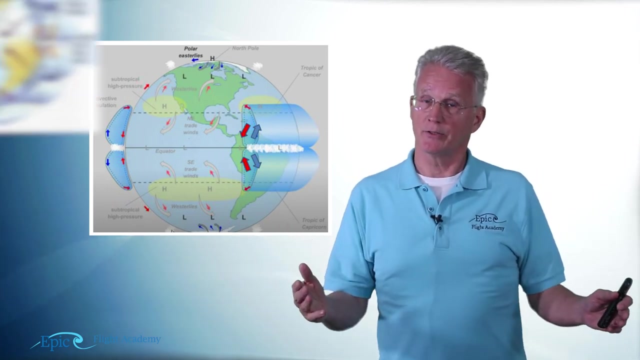 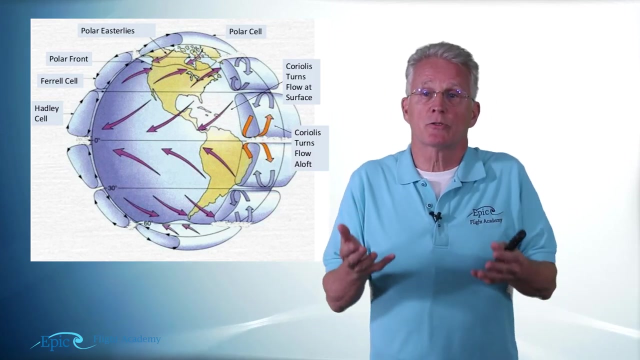 We also see Coriolis turning the aloft flow to the right, And that was that horizontal or flow parallel to the equator that we talked about with Coriolis force. Now that circulation creates what is called the Hadley cell At the equator, the air warms. As it rises, it starts to 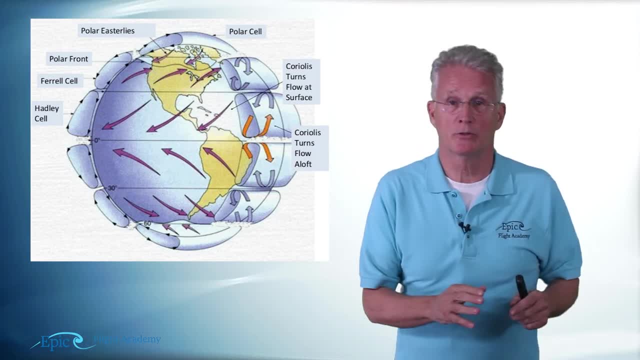 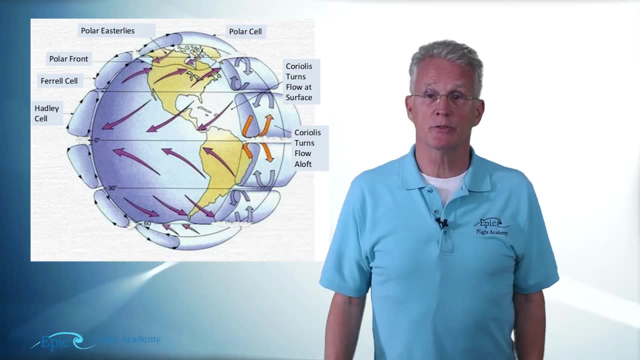 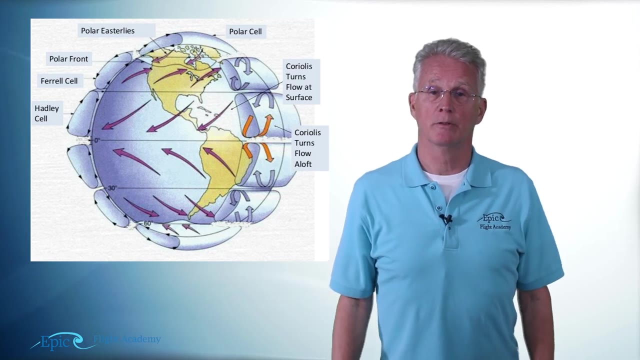 cool, losing moisture is deflected to the right, heading north aloft. It's moving over a smaller distance. It creates high pressure when it starts to sink near 30 degrees of latitude. And again Coriolis force is going to sink. And again Coriolis force is going to sink near 30 degrees of latitude. 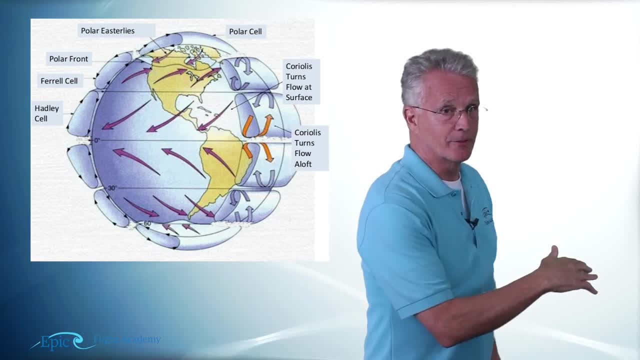 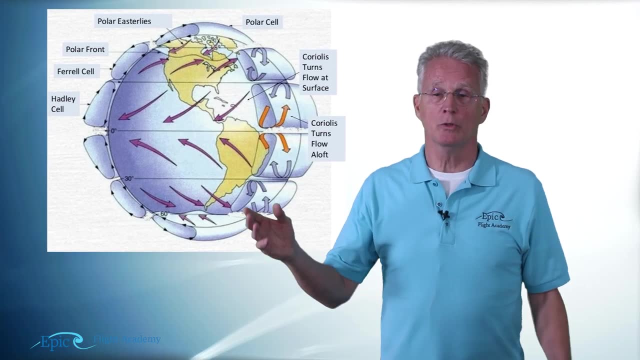 And again Coriolis force is going to sink near 30 degrees of latitude. And again Coriolis force directs it to the right at the surface- And these are called the trade winds- As it flows north and cools and dries and drops down at 30 degrees of latitude. 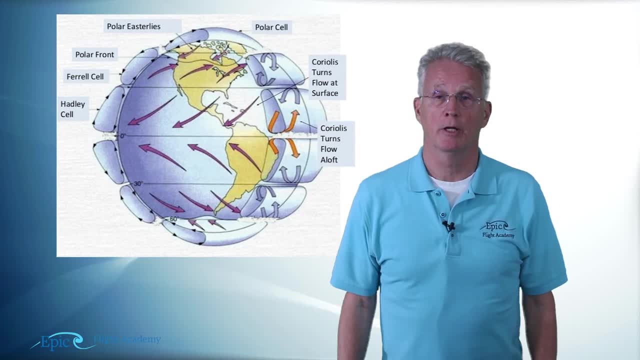 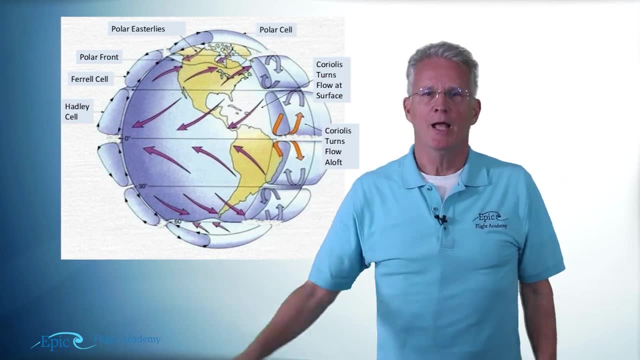 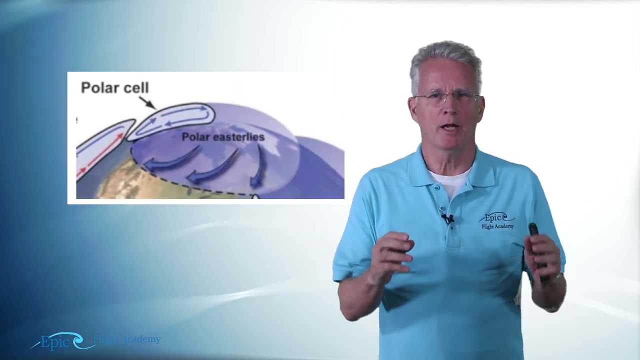 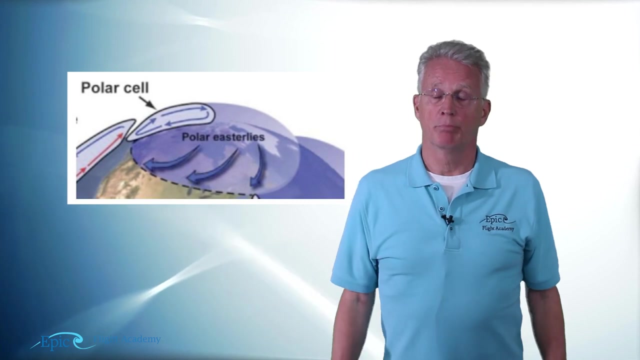 it creates these high pressure areas. Now let's jump from the Hadley cell all the way up to Santa Claus's house and let's go to the North Pole, The polar cold air sinks. Now remember back to our two vertical columns of air, red and blue. and we looked at why that cold air sinks and is more dense. As this cold air sinks and it starts to flow south, it is also warmed by compression And as it flows south, it starts to warm, and at approximately 60 degrees. 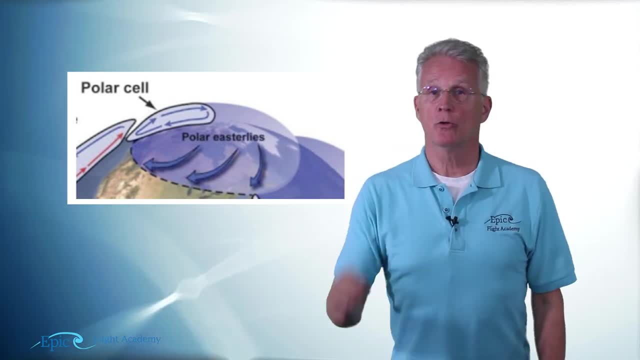 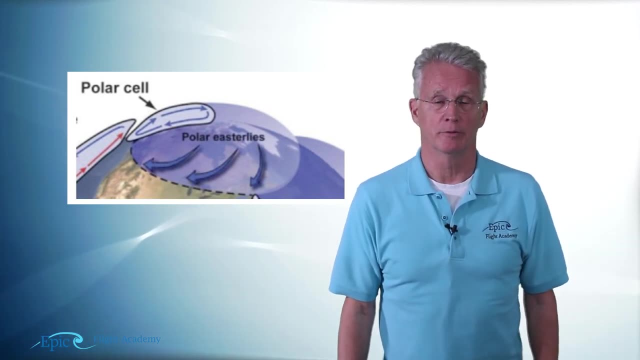 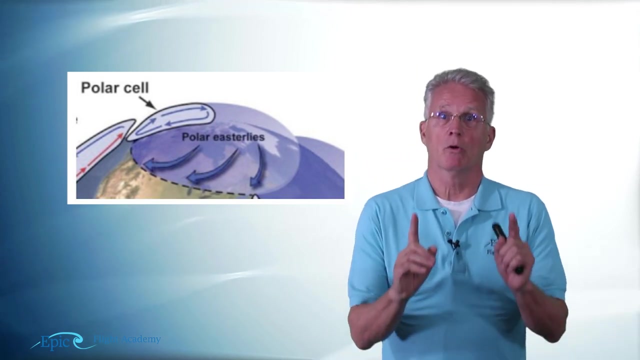 is ready to rise back up, creating predominant low pressure along 60 degrees of latitude. As it flows south from the pole, it is turned right in the northern hemisphere and the wind appears to come from the east. These are polar easterlies If it's flowing north from the south. 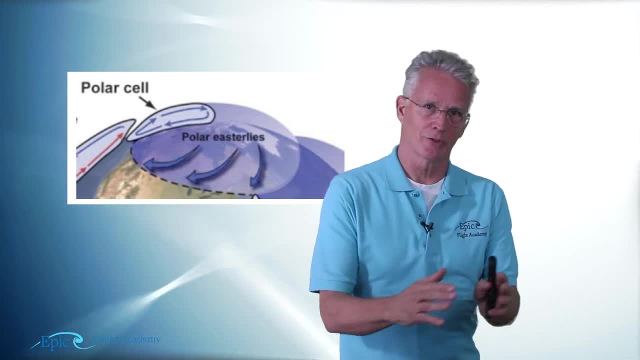 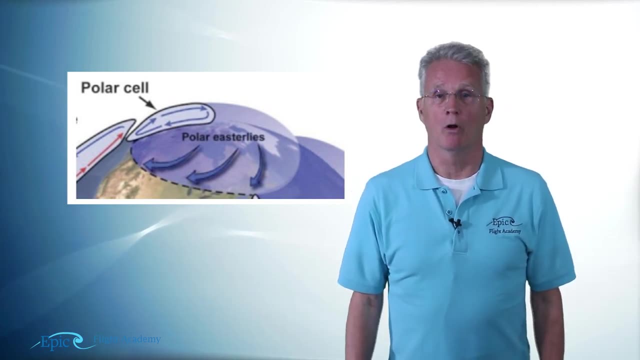 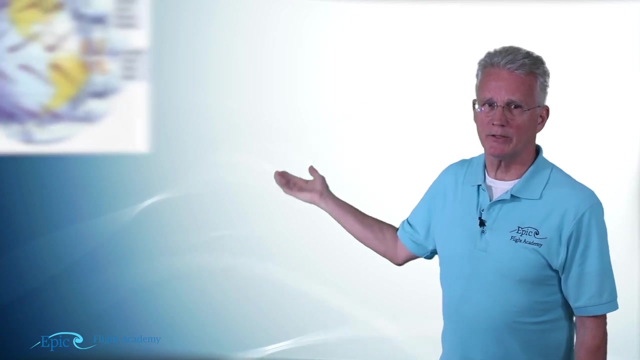 pole, Coriolis force turns it to the left Again. it appears to come from the east. So at the south pole we also have what we call polar easterlies. Now in our next diagram we start to see the whole. 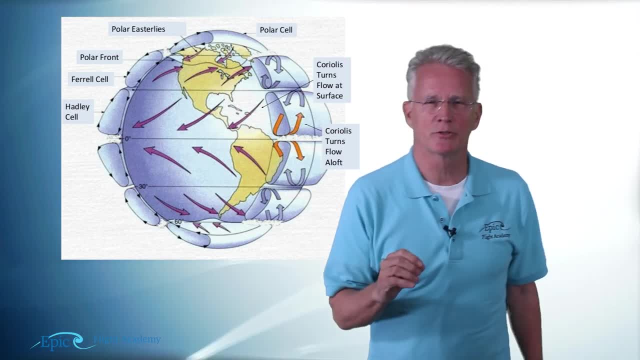 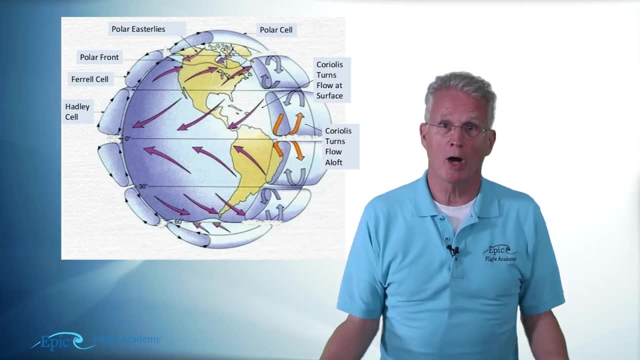 picture And I want you to notice something interesting: While air is sinking at about 30 degrees, it's not sinking at about 30 degrees. It's sinking at about 30 degrees. It's sinking at about 60 degrees of latitude And it's rising at about 60 degrees of latitude. This is causing low. 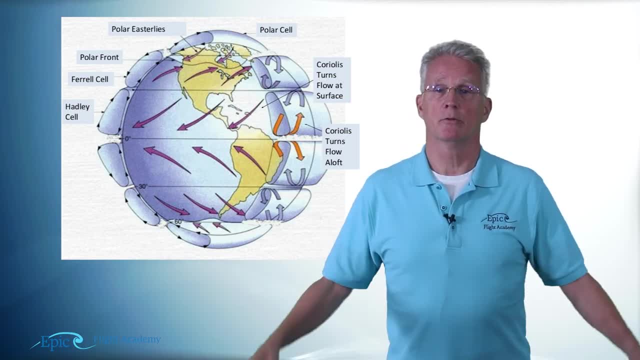 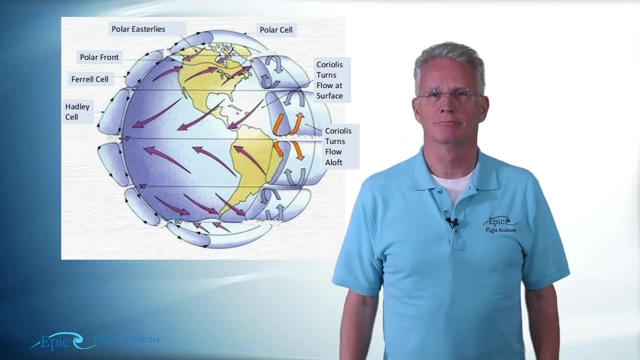 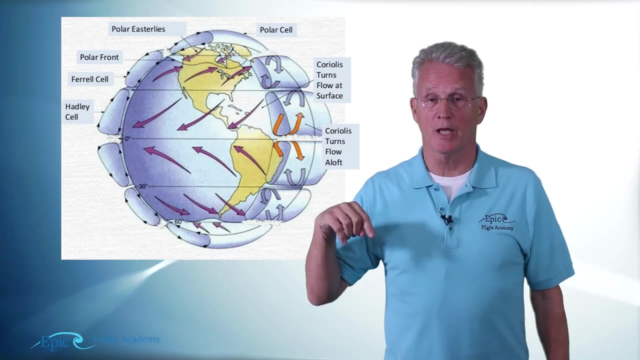 pressure at 60 degrees of latitude. higher pressure at 30 degrees of latitude. Now remember the pressure gradient force. The air will flow from high towards low, or in this case, from 30 degrees of latitude toward 60 degrees of latitude, And it's rising at about 60 degrees of latitude.